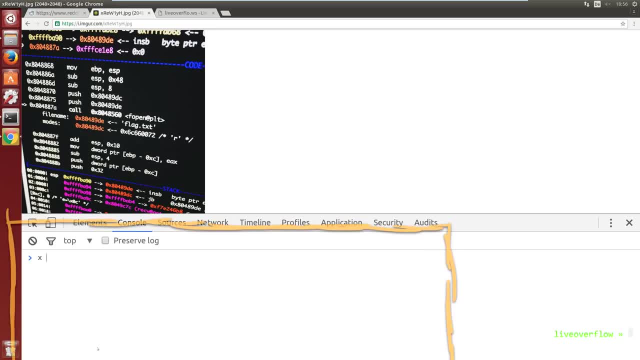 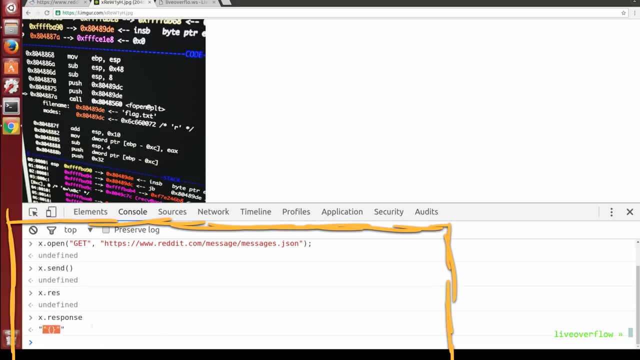 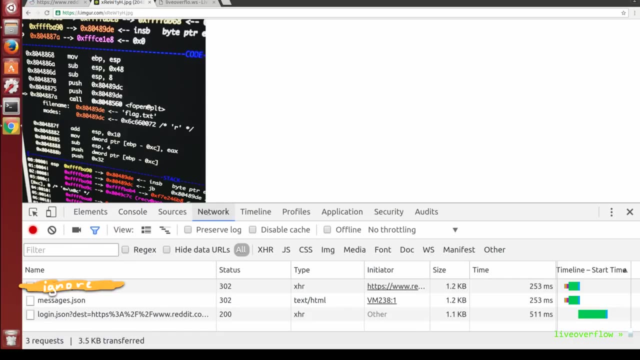 be able to get the content of this request as well. We can use xml http request to perform a get request. Looks like it worked, But the response is empty json And it doesn't contain the data we expected. Let's have a look at the network tab to see what happened. 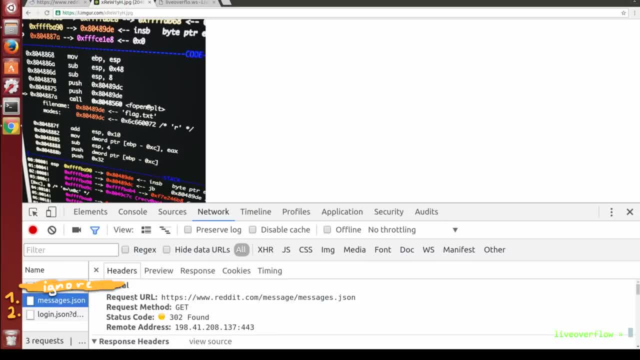 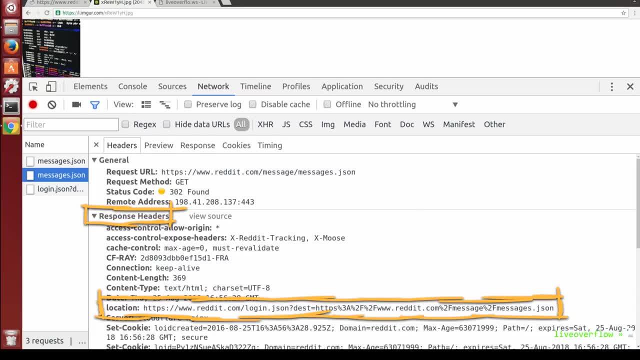 location header. The browser receiving this header will now perform a redirect to this new location, And this new location is slash login. Ahhhh, that makes sense. When we look closely, we don't see any cookies being sent along with this request, Like it did when we simply opened. 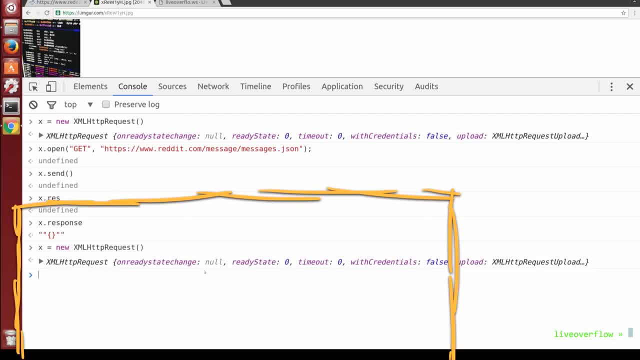 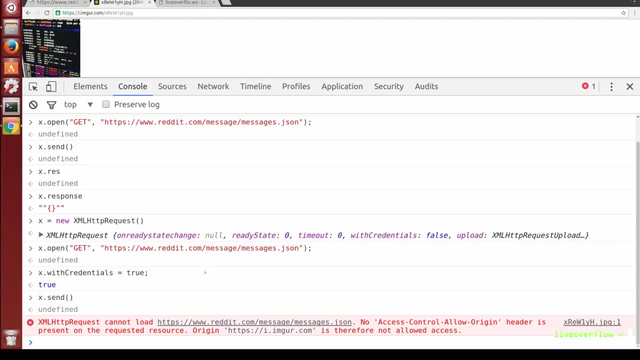 this url on reddit. A quick google search will tell you that you can include the cookies by setting with credentials to true before sending the request. But nope, Now it doesn't work. Now the browser complains that you are violating the same origin policy. 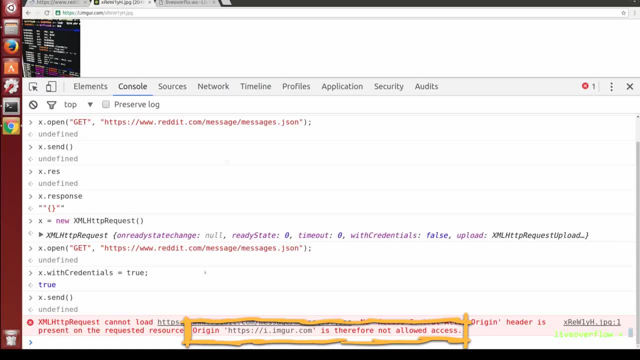 The domain imgorcom is not allowed to perform a get request to redditcom with cookies. This makes it kinda useless for an attack, Because as an attacker we would like to extract private user data. but without the cookies it will never contain private stuff. 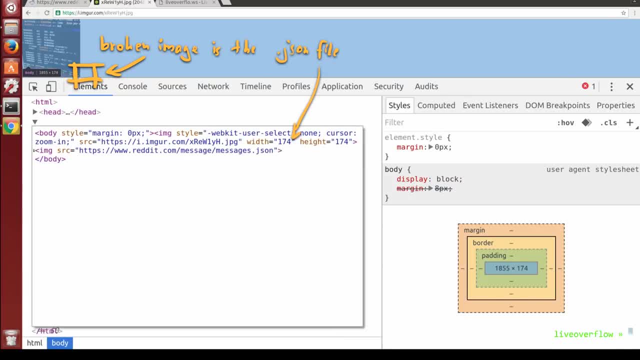 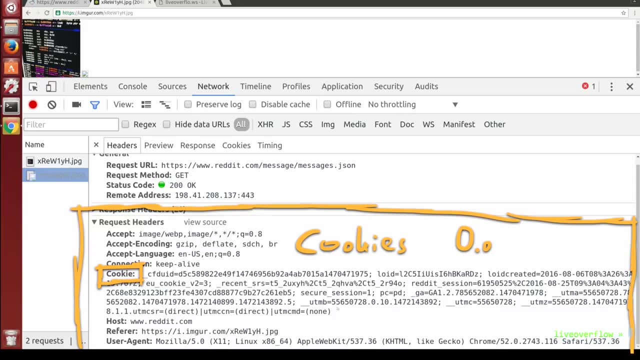 Let's try something else. Let's use an image tag, like earlier, and load this json file. We look into the network tab and… what the fuck? It did send the cookies with this request. So did we just find a bypass to the same origin policy? 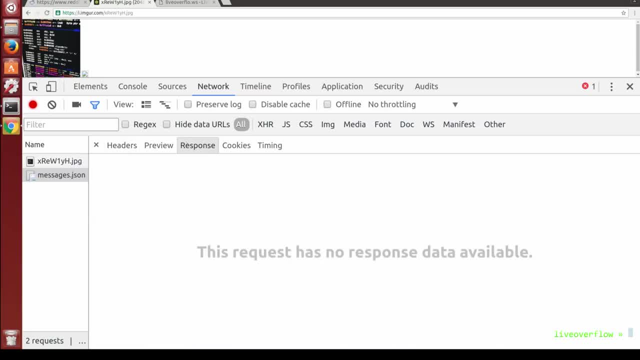 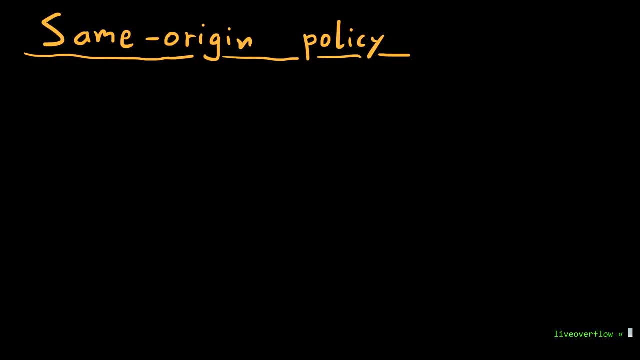 Well… no, You see, we can't access the response of this request. We cannot access the json content. thus we cannot access the private user data. Ok, so it looks like the same origin policy is pretty good. It prevents us from accessing private data across origins. 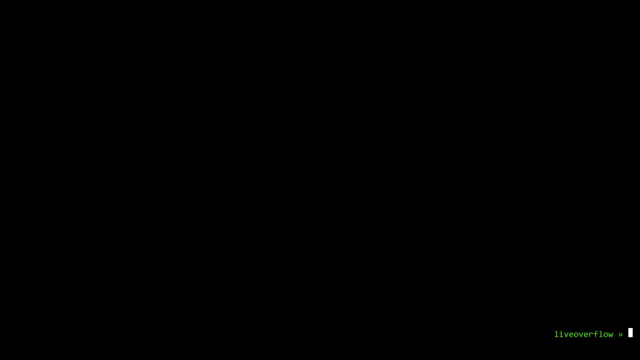 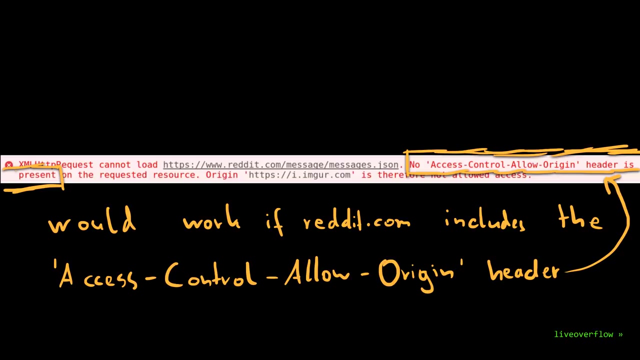 Of course, there are some technical possibilities to loosen up this policy, And chrome even tells you about it in the description of this video. If you want to learn more about this, check out the link in the description With this special response header that could be set by the reddit server. 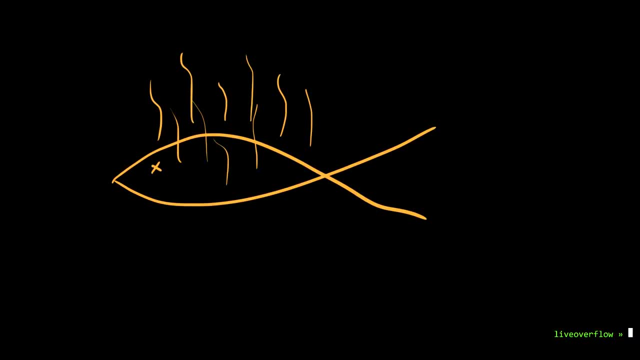 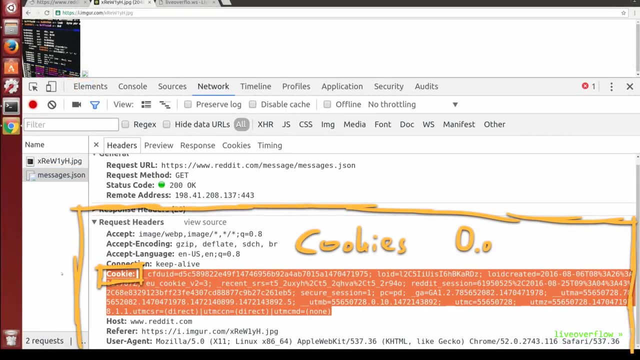 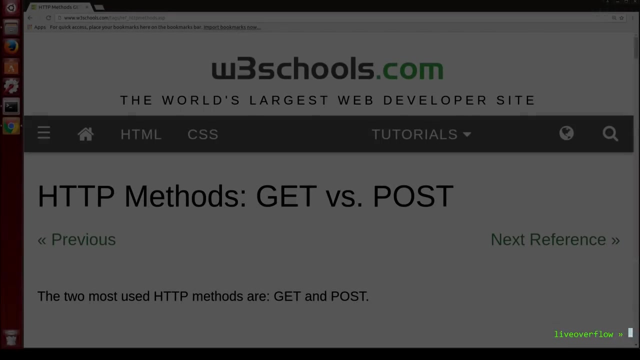 this could be allowed. But one thing is still fishy With the image source. we just performed an authenticated, meaning cookies were included request to the other domain. We don't get the response, but could this still be exploited in a meaningful way? Yes, it can. Let's see. You remember the different HTTP methods. 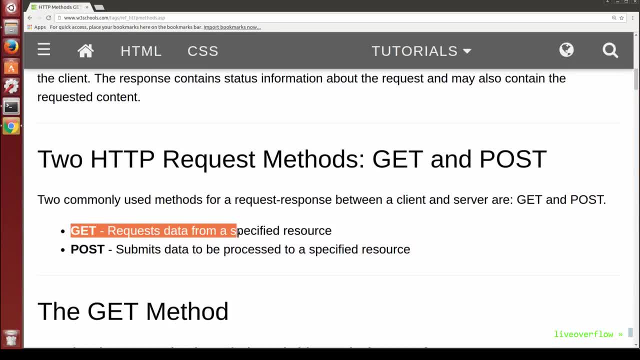 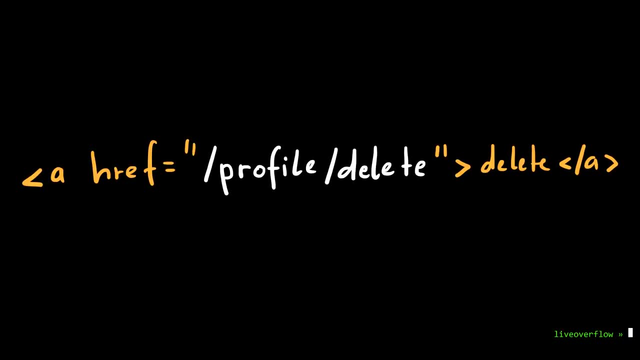 like GET and POST. Generally, GET requests are intended to fetch, to GET a resource and nothing else, While POST requests potentially change a user's data. So performing an authenticated GET request should generally be safe, except when a site is developed badly and a URL is accessible. via GET performs an actual action. If that is the case, you have found 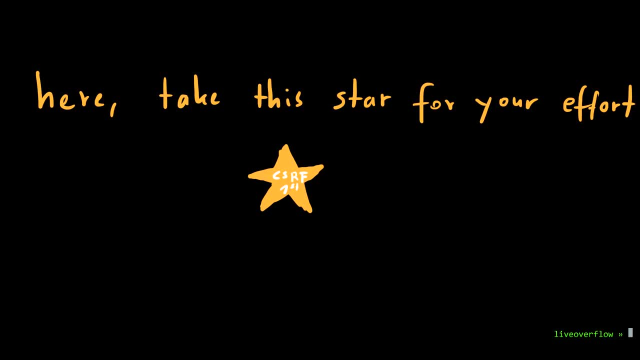 your first cross-site request: forgery CSRF vulnerability. So if there is, for example, a URL that deletes a user like profile delete, you can use this method to get the response to the user. So if there is, for example, a URL that deletes a user like profile delete. 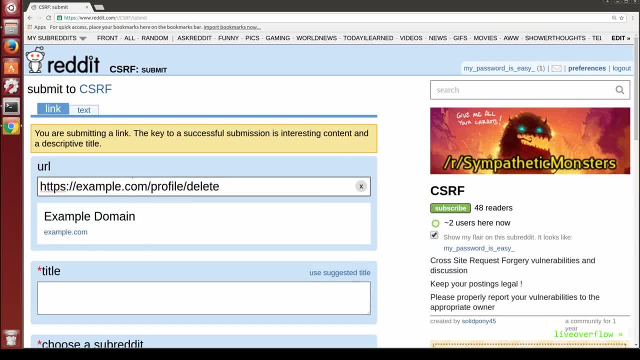 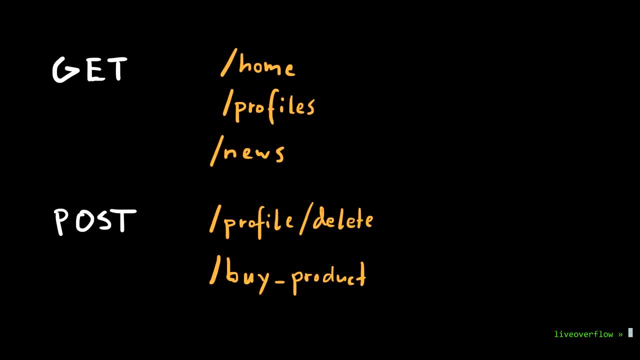 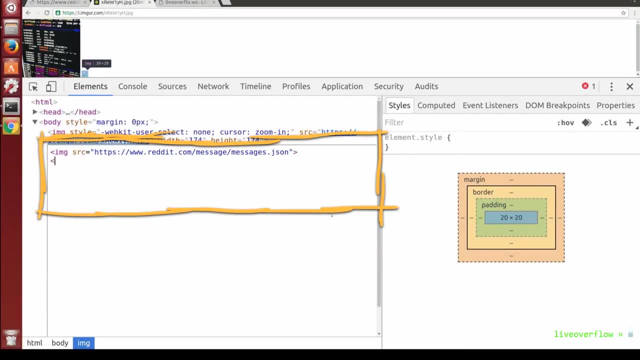 you embed that as an image on your website, then every user visiting your site will delete their profile without them noticing it. Ok, But let's say the developer follows this design and there are no state changing GET requests. Is this site safe? Well, here is another technique for POST requests. I can create a form with the method POST and the 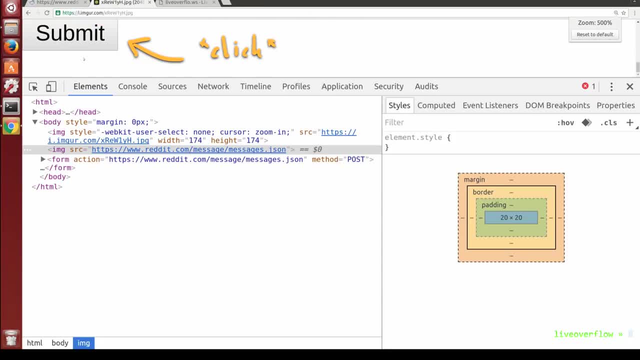 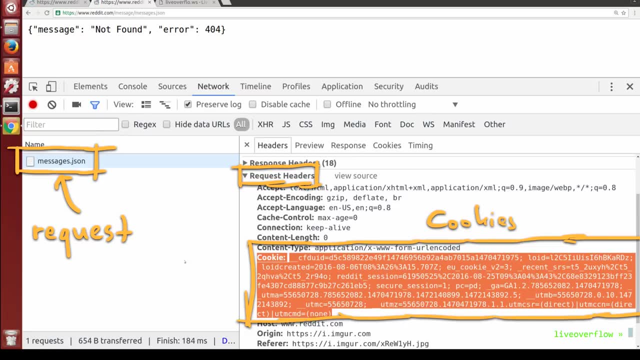 action aiming at the other domain And when we submit the form, it will perform a POST request with the cookies. So, yes, we can perform an authenticated POST request as well, Though the site also redirects to the other new domain. but we can hide that from the user or don't care. 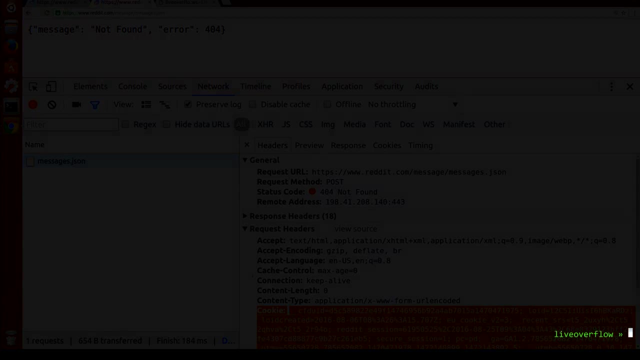 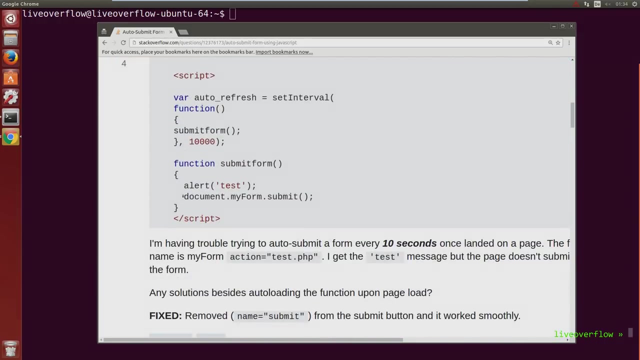 because the attack then is over anyway. But how do I get a user to click? Well, a user doesn't have to click. you can simply autosubmit this form with javascript. Just to make it clear: the same origin policy is not violated here, because our origin does not get to access the. 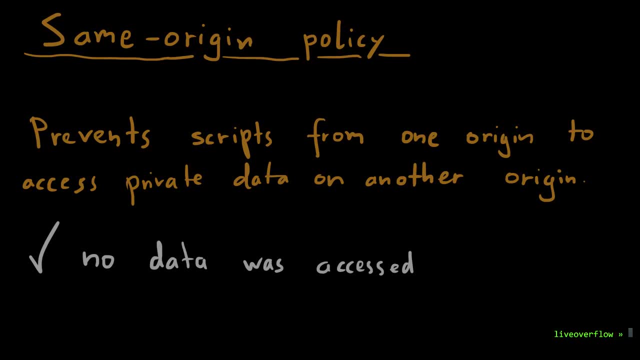 resources to the user. So if you are using a POST request, you can submit this form with the same POST request, but this will only protect the data of this other domain. So how do we protect from this kind of attack? One approach would be to compare a legitimate 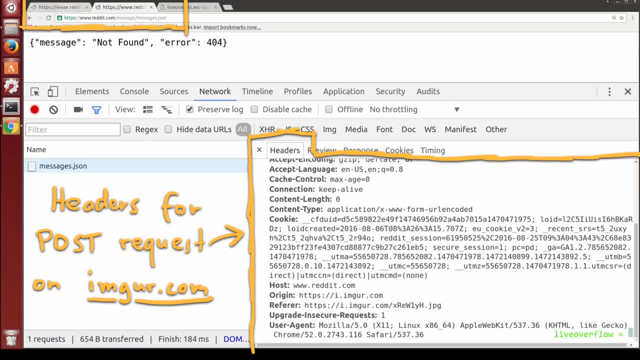 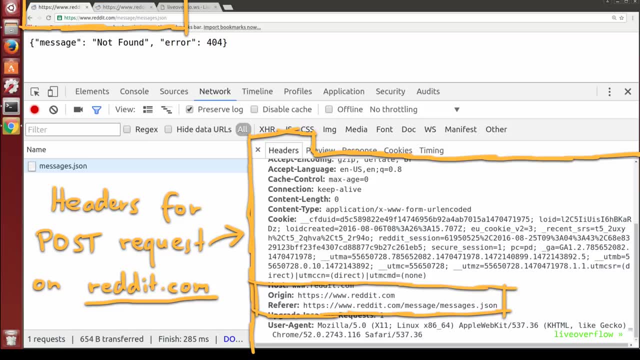 request from our domain with an illegitimate request from another domain and see if there are any differences that we could check for. And yeah, we could check for the origin header, Which is definitely different. This might sound like a good idea. It certainly prevents some. 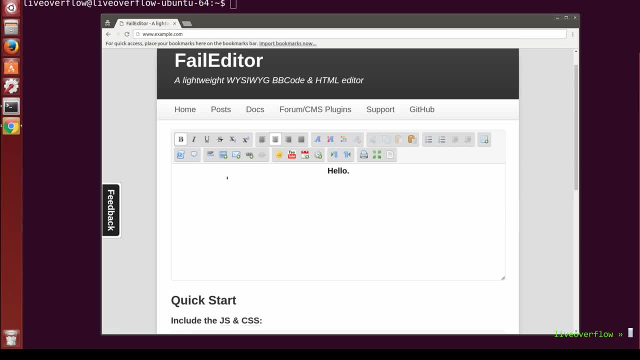 kind of cross site request forgery attacks. But, for example, sites like forums allow you to do this. If you want to get a clash with a domain, you can do that here, But if the users to embed their own pictures and if this forum is vulnerable to a get-csrf attack, 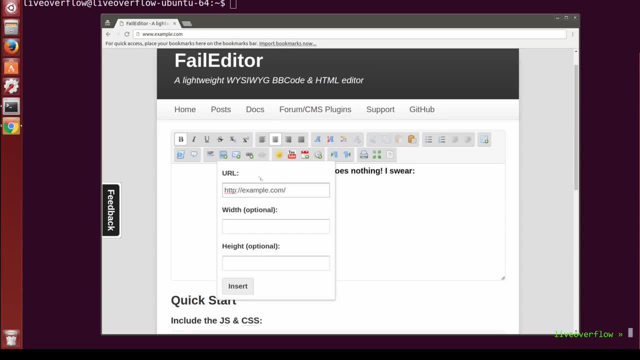 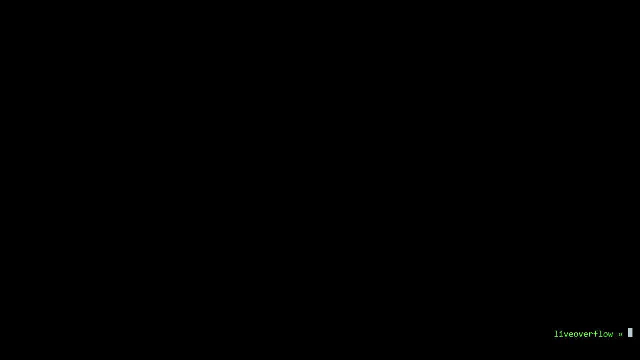 then users could simply embed that url as an image into a message and then the request would come from the same domain. So this is not a bulletproof protection. There are also some kind of mitigations. for example, form-post requests always send the. 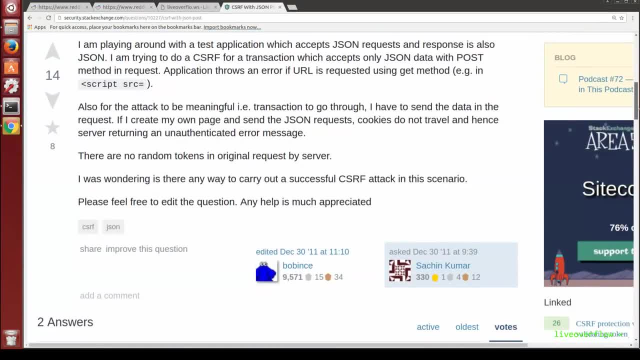 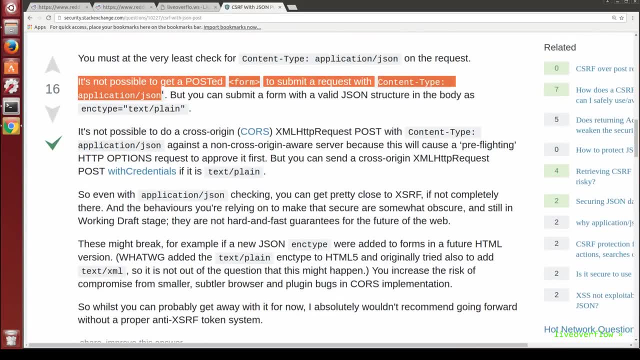 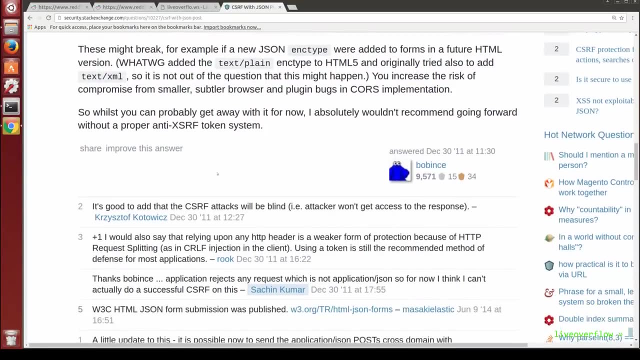 data url encoded And you may have found this old stack-exchange thread telling you that a cross-domain request with the content type json is impossible and your endpoint could only accept json data and this might prevent some noobs from exploiting it. But your trust into this protection is flawed. 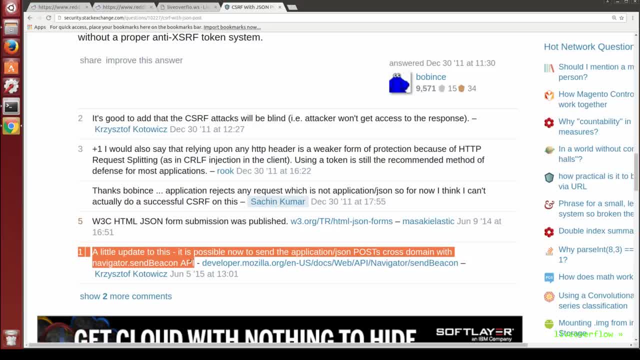 Down here in the hidden, in a comment, you find information about a trick using navigator send beacon. It's a super awesome trick, And little tricks like that make the difference between a normal web penetration tester and a great one. Anyhow, as you can see, this is also not bulletproof. 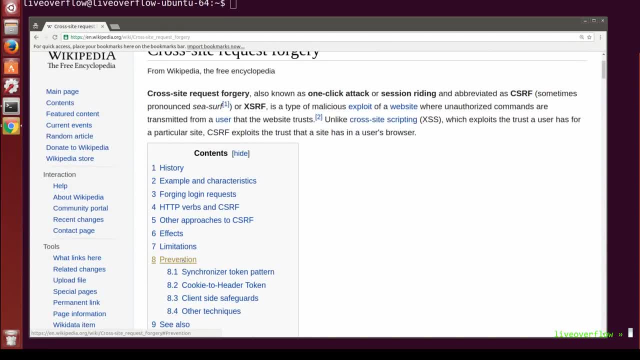 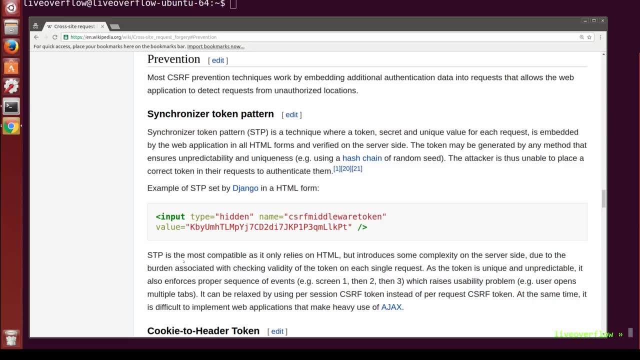 So then, what can we do? The solution is called CSRF token. CSRF tokens can be implemented in a few different ways, but generally you want a secret random value to be set by the server in a way that it's only accessible to the website running. 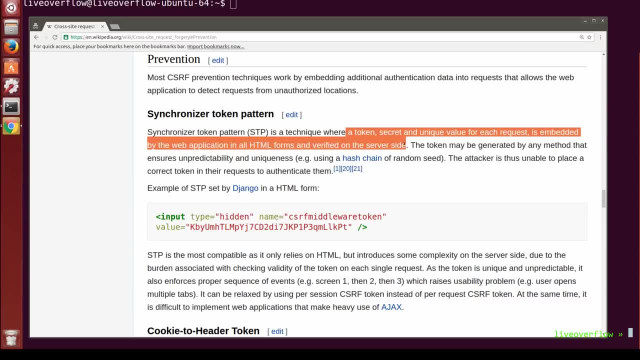 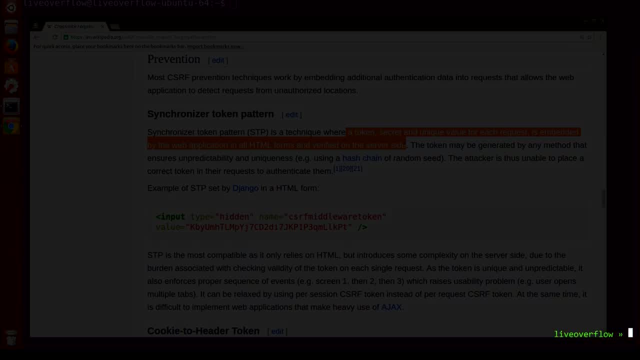 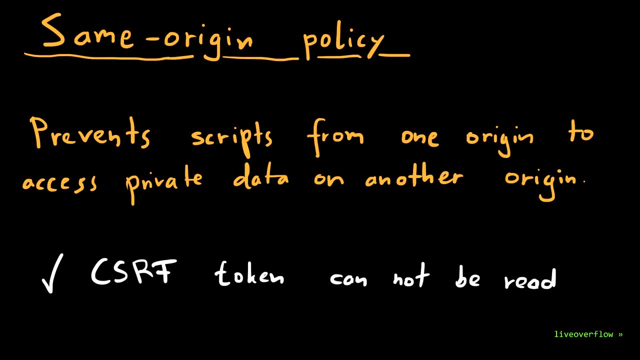 on the same domain And this secret value has to be included in every post request to the server, Otherwise it will refuse to react to the request. And that works Because the same origin policy prevents other domains accessing your data. this cannot get the secret CSRF token, but the legit domain can. 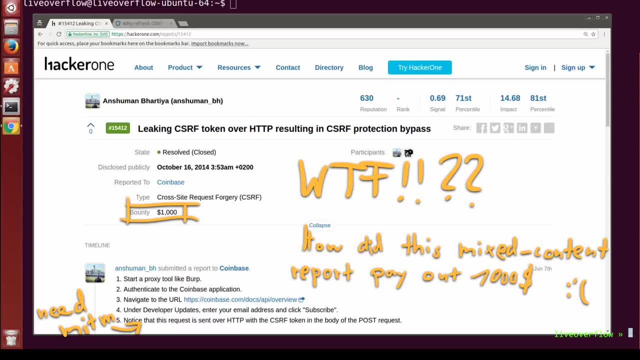 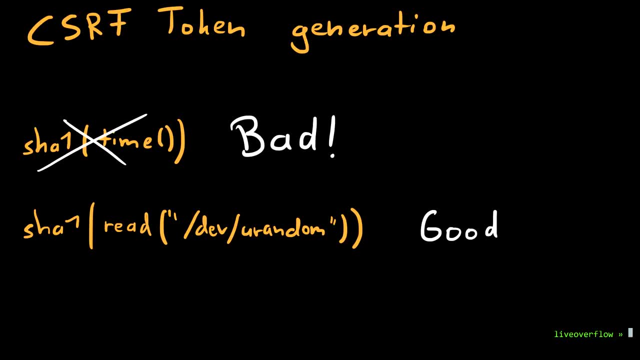 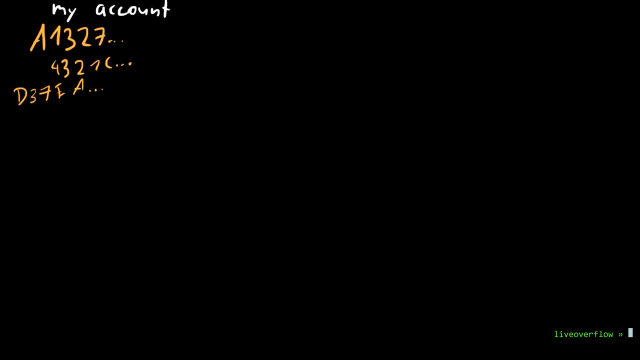 Obviously, if you find a way to leak the CSRF token, then you defeat the CSRF protection. Now, this token doesn't have to change with every request, but the idea is that it's hard to predict, So it shouldn't be valid forever. Also, very, very important, CSRF tokens have to be bound to your users session. 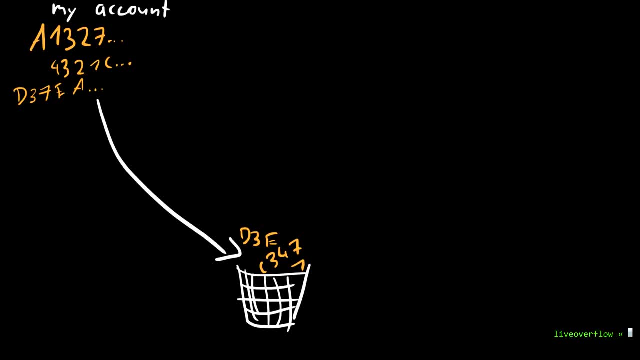 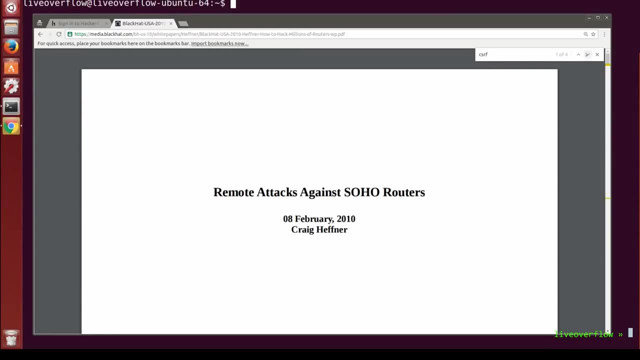 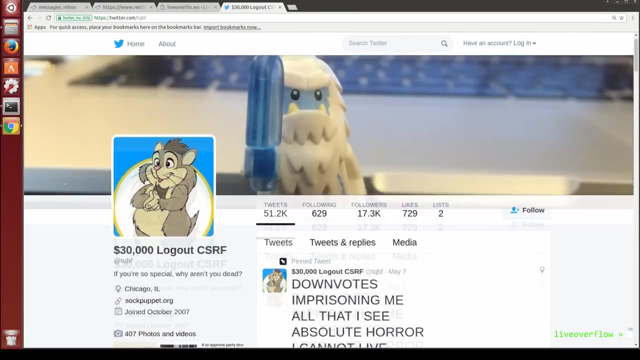 Otherwise, I could, for example, collect valid CSRF tokens with one account and then use them in a CSRF attack against other accounts. Cross-site request forgery can be extremely powerful and bypassing a weak CSRF protection can be super fun. But make no mistake: just because a website has a vulnerable endpoint doesn't mean it's.